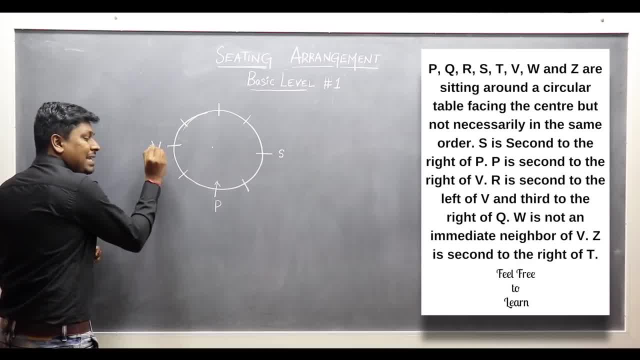 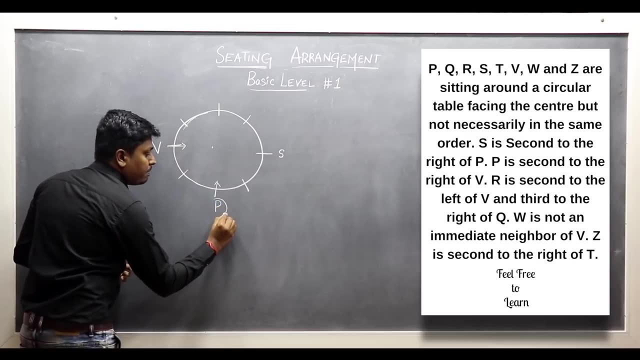 because we know all the persons are facing a center. Only, if I fix V here, we know V is facing center and V right hand side will be this side and V left hand side will be this side. So, according to the point V- right hand side, at a second place, P is sitting. So now I confirm that P is sitting. 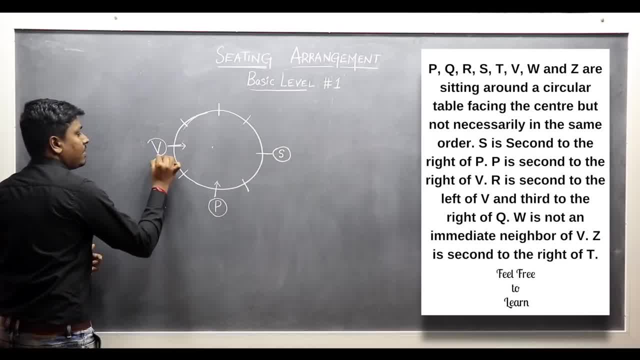 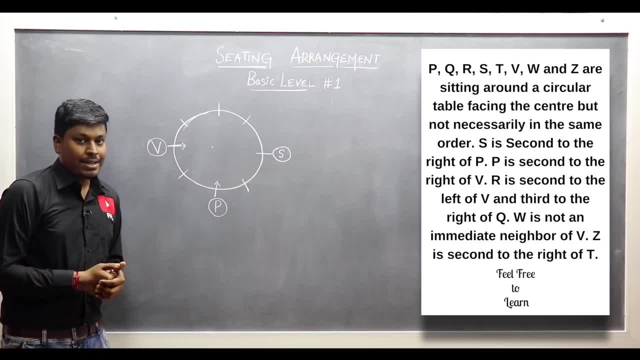 here, S is sitting here and also V is sitting here. So these are the points I have confirmed. So next point: R is second to left of V, So V, left hand side at a second place. who is sitting? R is sitting. We already fixed V here. We know V right hand side will be this side and left hand. 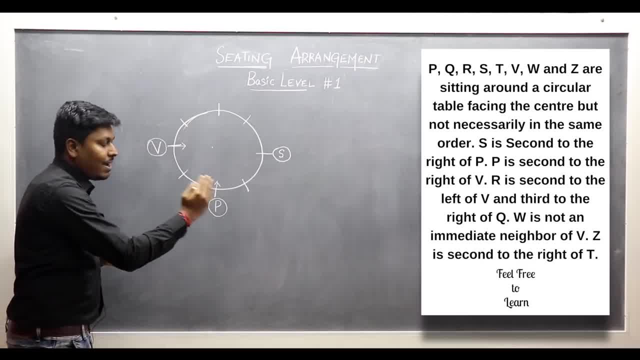 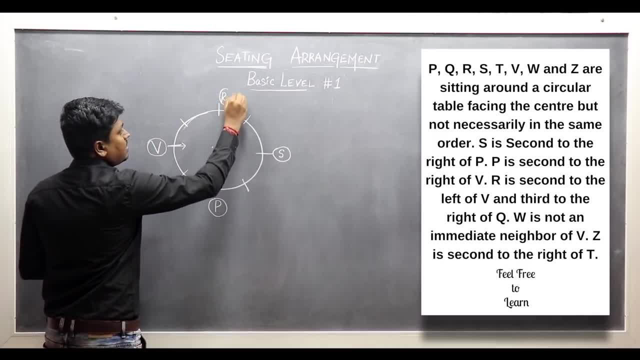 side will be this side. So now, according to the point V, left hand side, at a second place R is sitting. So first place and this will be the second place where R is sitting. So this is the place for R. Next and third to right of Q. 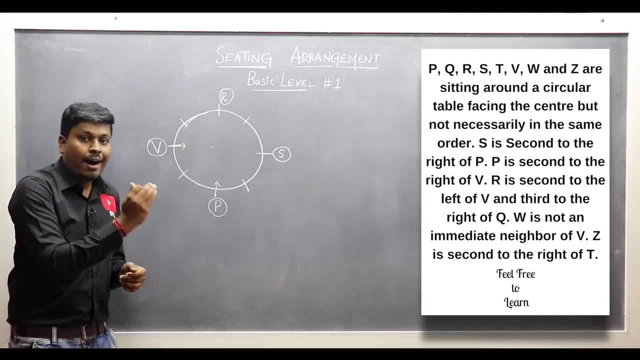 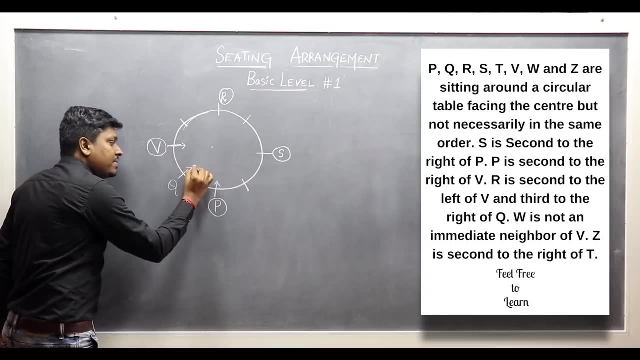 So Q right hand side at a third place where R is sitting. So remember that Q right hand side at a third place who is sitting? R is sitting Where you need to fix Q. See here. if I fix Q here, for example, I am saying if I am fixing Q here, we already know that everyone is facing the center. 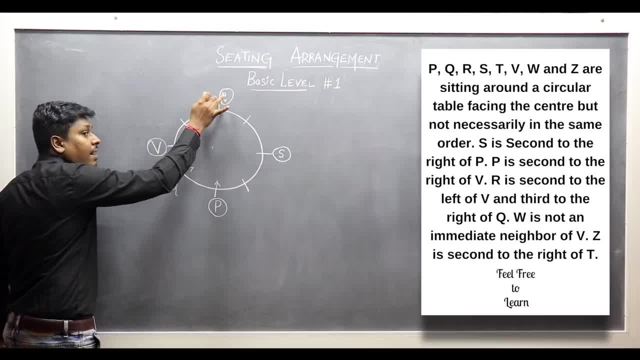 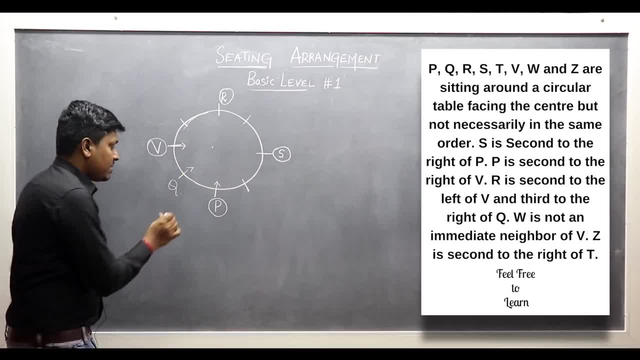 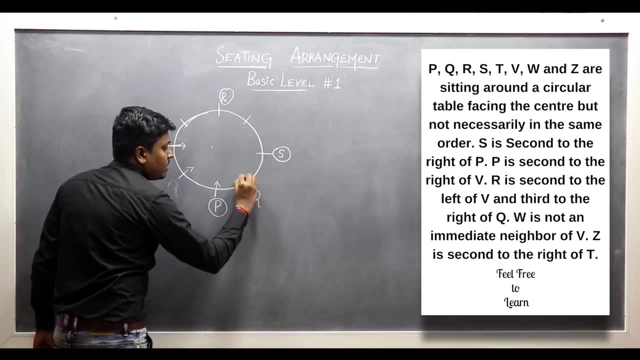 So Q, left hand side, at a third place is R according to this diagram. But what actually the question says, Q, right hand side, third place should be R. So definitely I should not fix Q here. I should fix Q here. So Q and Q is facing center Only then according. 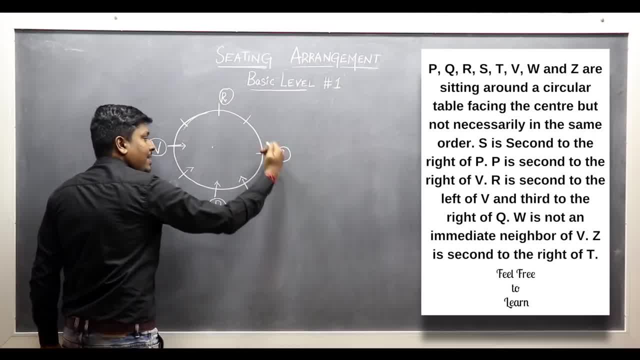 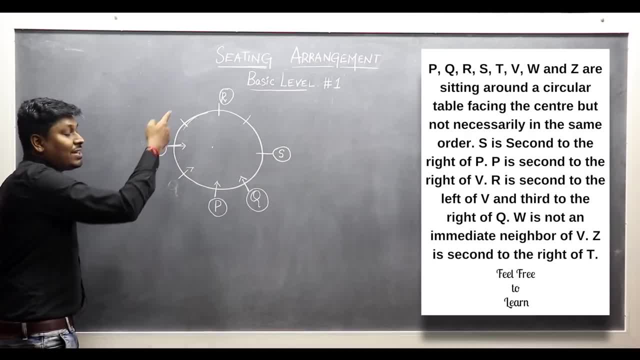 to the question. the diagram will be correct Because Q right hand side at a third place is R. So finally, I fixed Q. In case, if I fixed Q here, then Q left hand side, third place will be R. According to the question, Q right hand side, third place should be R, Got it? 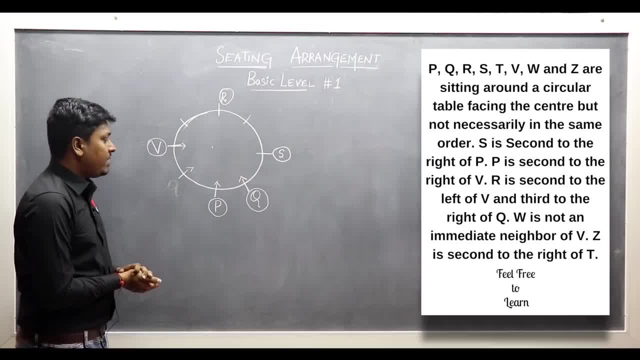 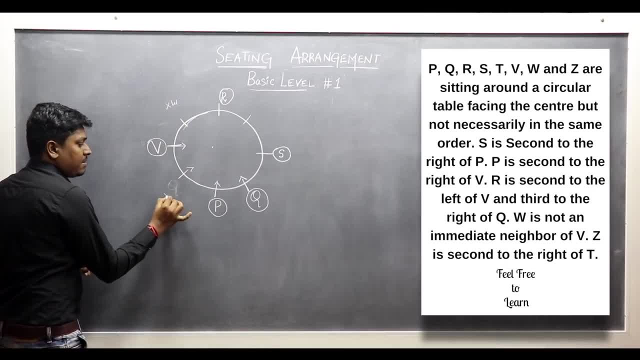 Next point: W is not an immediate neighbor of V, So V immediate neighbor is not W right. So V should not fix W here. It is not the place. And similarly I should not fix W here because V immediate neighbor. both these places should not be W. Then only one place is remaining.